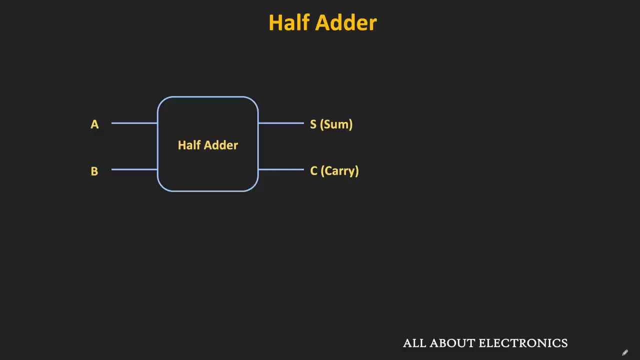 and the carry bit as the output. So now let us see what is the logic circuit of this half adder, And for that using the truth table. first of all, let us understand that when we add the two bits, then what are the possible outcomes? 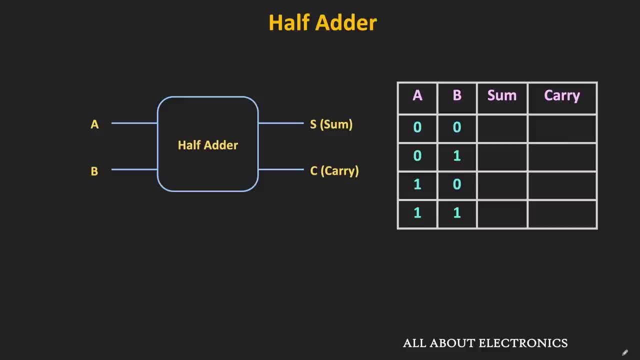 So for the two bits there are total four different combinations, right? So here this 0 plus 0 is equal to 0. That means, whenever this a and b is equal to 0, then the sum bit and the carry bit both. 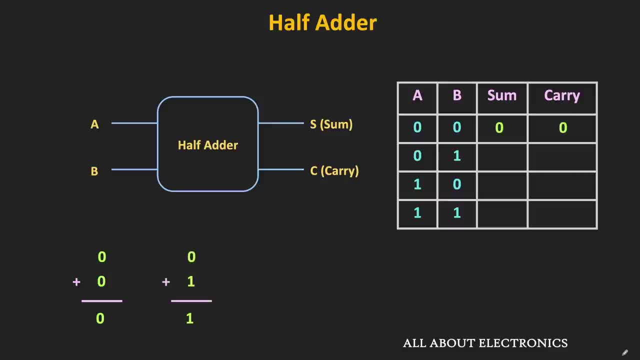 are equal. Similarly, this 0 plus 1 is equal to 1.. That means this sum is equal to 1 and the carry is equal to 0. Likewise, this 1 plus 0 is equal to 1.. That means whenever this a is 1 and the b is 0, then this sum bit is equal to 1, and. 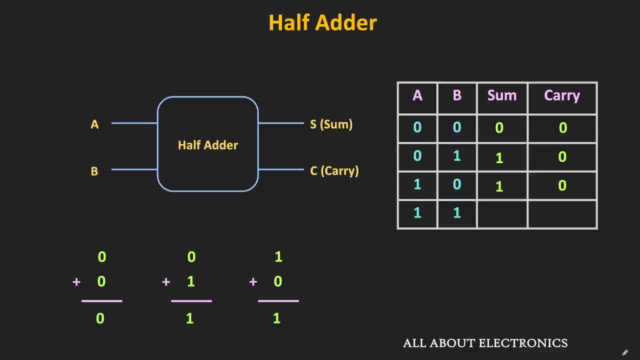 the carry bit is equal to 0. And likewise this 1 plus 1 is equal to 0, with 1 as a carry. That means, whenever both a and b is equal to 0, then the sum bit is equal to 1 and the 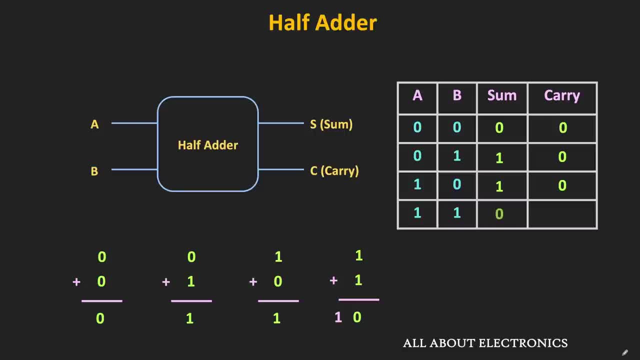 carry bit is equal to 0. Then this is the truth table of the half adder. So this is the truth table of the half adder. So you see both of them. So, as you can see this sum output is equal to 1 when a is 0 and b is 1.. 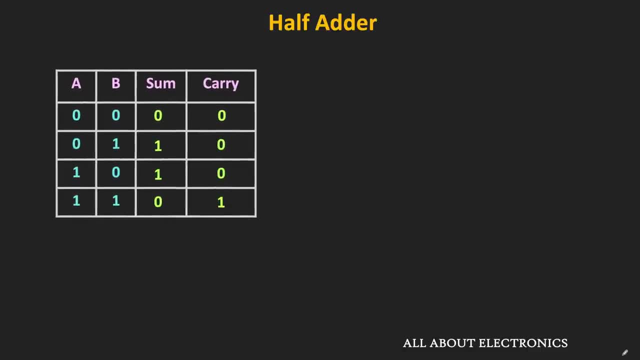 Or when a is equal to 1 and b is equal to 0. So if you see the Boolean expression of this sum output, then it is equal to a bar dot b plus a dot b bar, Or it is equal to axor b. 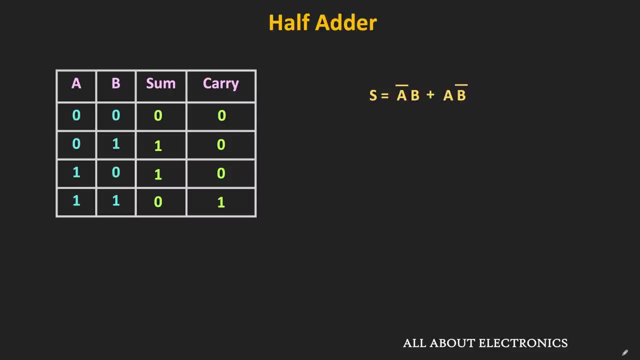 So for the next совir, I will always write denominators for b. We also have máquina's clues. We haven't brought them here yet. Similarly, this carry bit is equal to 1 when both A and B is equal to 1.. 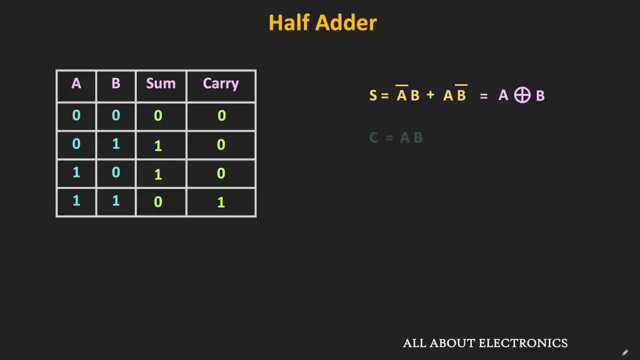 Therefore, if we see the Boolean expression of this carry bit, then it is equal to AB. So these are the Boolean expression of the sum and the carry. So now let us implement them using the logic gate. So, as you can see these expressions, the sum output can be implemented using one 2-input. 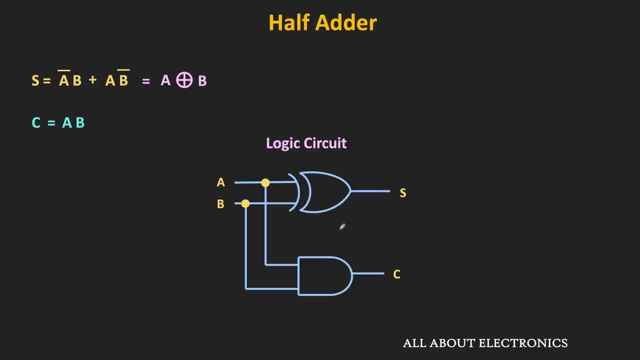 XOR gate, while the carry output can be implemented using one 2-input AND gate. So this is the logic circuit of the half adder. Now this half adder circuit works perfectly when there is no incoming carry. But if there is an incoming carry from the previous addition, then we cannot add that. 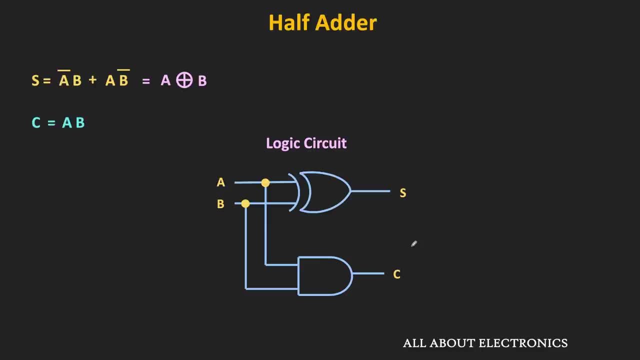 carry using this half adder. For example, let's say we want to add these two binary numbers. Now the LSBs of these two numbers are 1 and 1. So these numbers can be added using the half adder because during the addition there is 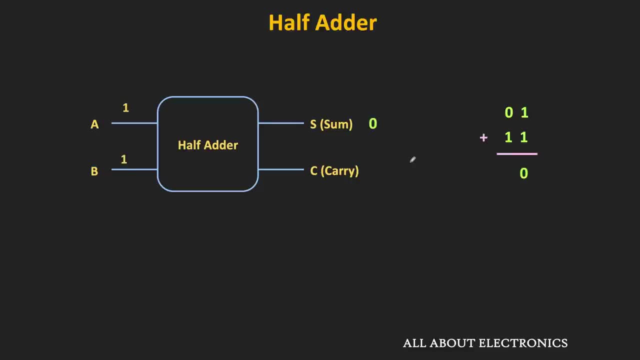 no carry. So after the addition this sum bit is equal to 0 and the carry is equal to 1.. So now in the next column, if you see, then we have the carry bit along with these two bits, And this carry bit is generated from the previous addition. 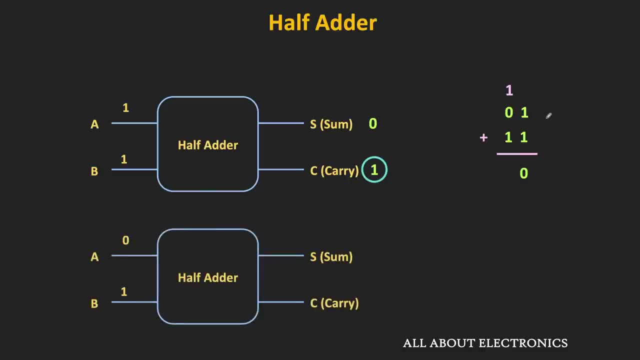 So if we try to do the addition using the half adder, then simply we need to ignore this carry bit And that is the limitation of this half adder. That means using the half adder we cannot add the carry which is generated from the. 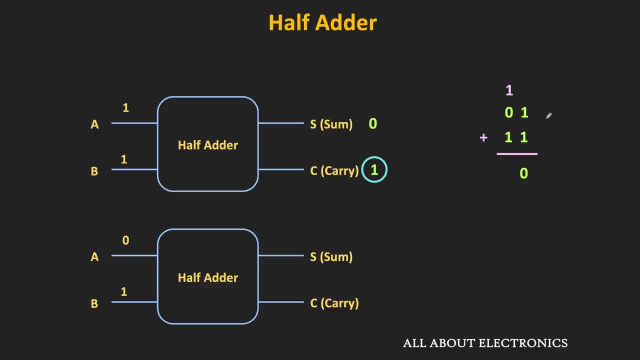 previous addition. So if we want to do the addition of the two bits along with the carry bit, then it can be performed using the full adder circuit. So this full adder is the combinational circuit which adds the two bits and the incoming carry. 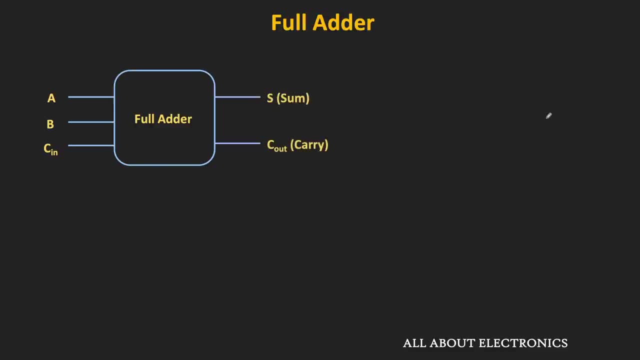 bit and generates the sum and the carry bit as the output. So now let's see the logic circuit of the half adder. Let's see the logic circuit of the half adder. Let's see the logic circuit of this full adder. 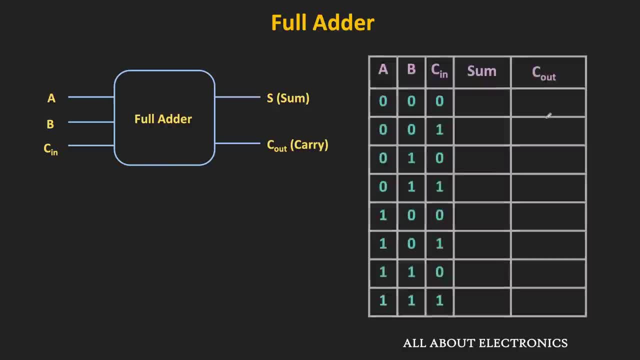 And for that first let us see the truth table of this full adder. So here for the three inputs, we have total 8 different combinations, right? So here in the first row, this 0 plus 0 plus 0 is equal to 0.. 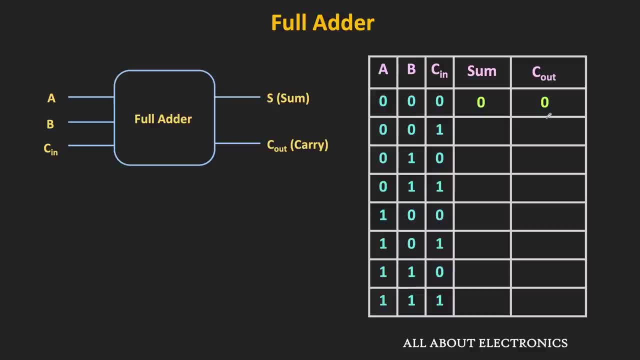 That means the sum is equal to 0 and the carry bit is also equal to 0. Similarly, in the next row, this 0 plus 0 is equal to 0.. And then this 0 plus 0 is equal to 0.. 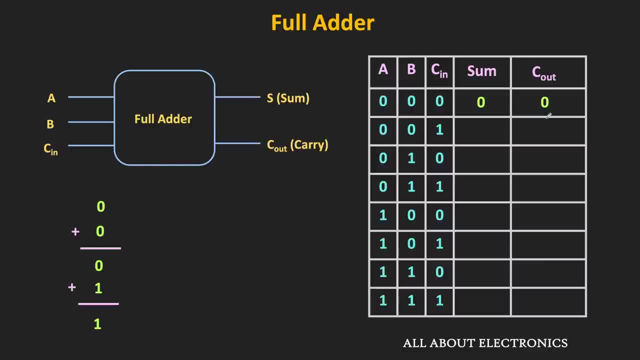 So in this first row the sum is equal to 2 and the carry bit is also equal to 1.. Product: divide this into two动ü引. Then in the second row, this 0 plus 1 is equal to 1 and the carry bit is also equal. 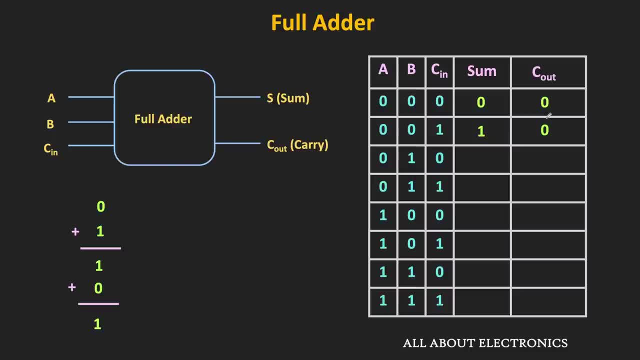 to 0.. Since the number is 1, it is crucially equal to 0. That means, in the third row, the sum is also equal to 1 and the carry bit is also equal to 0.. Likewise, in the fourth row, this 0 plus 1 is equal to 1 and this 1 plus 1 is equal to. 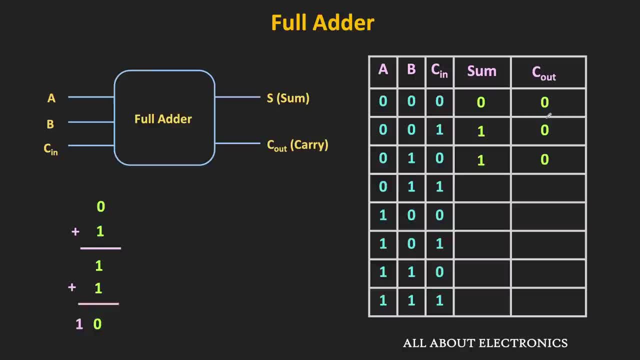 0, with 1 added a carry. That means in the 4th row, the sum bit is equal to 0, while the carry bit is equal to 1.. Likewise, in the 5th row, this sum bit is equal to 1,, while the carry bit is equal to 0.. 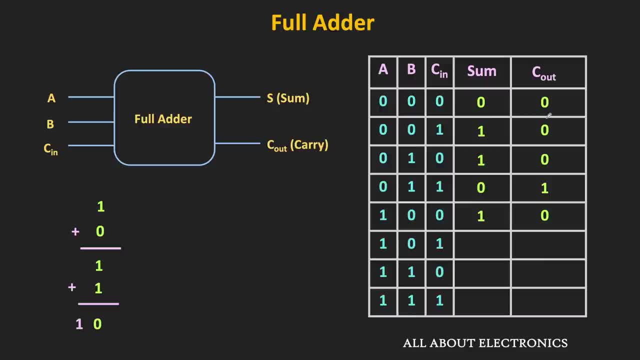 And similarly in the 6th row, 1 plus 0 is equal to 1, and the 1 plus 1 is equal to 0, with 1 as a carry. That means the sum bit is equal to 0,, while the carry bit is equal to 1.. 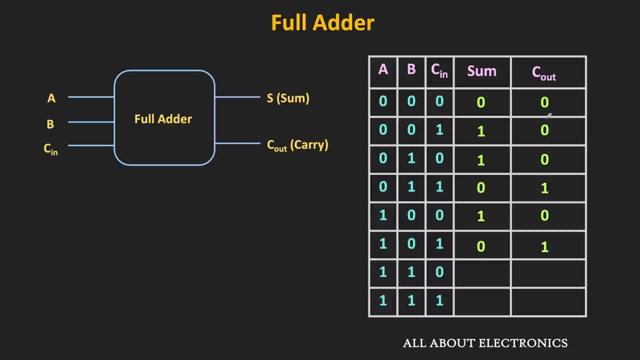 Similarly, if we see the 7th row, then in this row 1 plus 1 is equal to 0, with 1 as a carry, And then this 0 plus 0 is equal to 0. That means, here the sum bit is equal to 0, while the carry bit is equal to 1.. 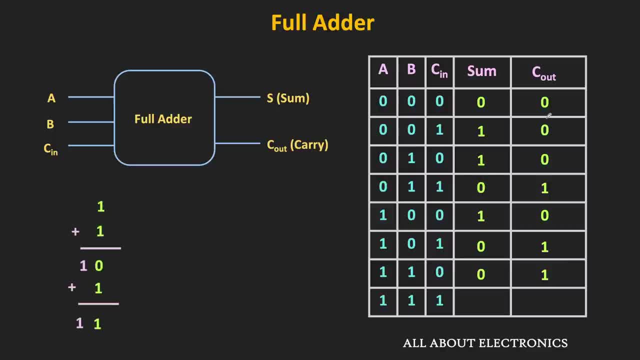 And finally, in the 8th row, 1 plus 1 is equal to 0, with 1 as a carry, And then this 0 plus 1 is equal to 1.. That means in the 8th row the sum bit is equal to 1, and the carry bit is also equal. 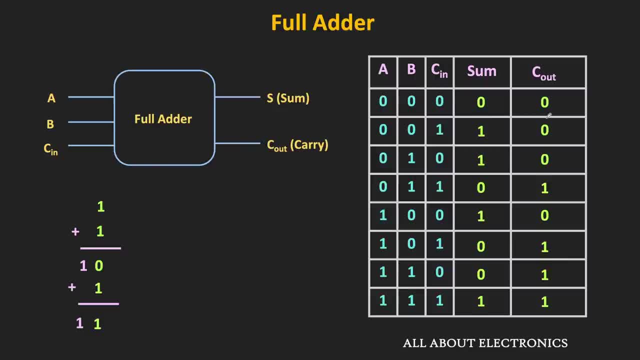 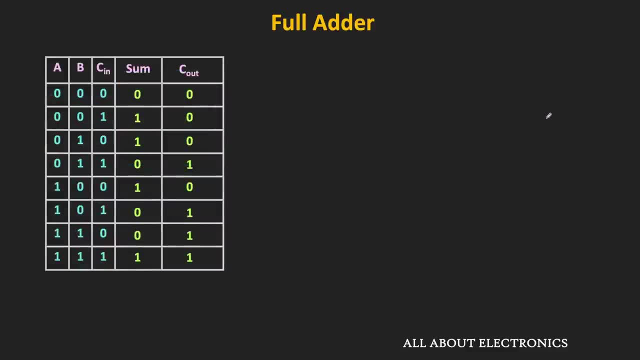 to 1.. So in this way we got our truth table for the full adder. So, as you can see, this sum bit is equal to 1 for the 4 different input combinations, And likewise this carry bit is also equal to 1 for the 4 different input combinations. 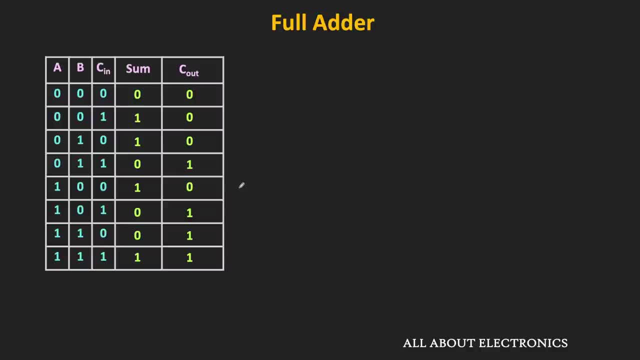 So now let's find the Boolean expression of this, The sum bit and the carry bit, And then let's try to minimize them. So, as I said, this sum output is 1 for the 4 different input combinations. And this is the Boolean expression of the sum output. 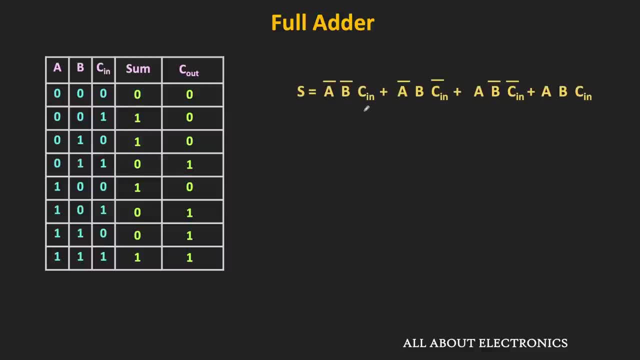 So now in the first two terms, if we take this a bar common, then in the bracket we will have this: b bar dot sin plus b dot sin bar, And that is equal to bx of sin. Similarly, In the last two terms, if we take this a common, then in the bracket we will have: 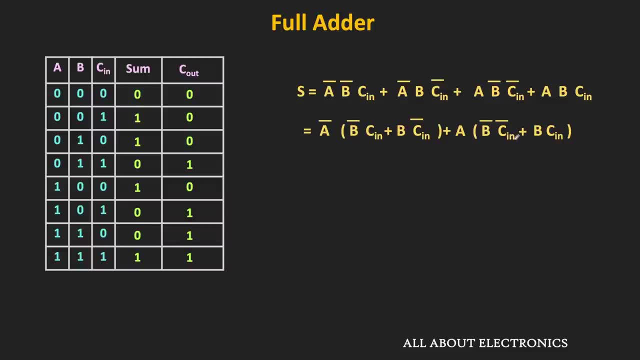 this: b bar, dot sin bar plus b dot sin, And this is equal to bx nor c, or that is equal to bx or c whole bar. That means we can write this expression as a bar dot bx or sin plus a dot bx or sin. 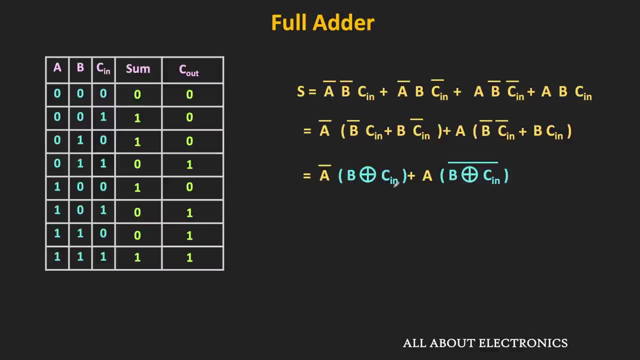 whole bar. Now let's say this: bx or sin is equal to x. That means we can write this expression as a bar dot x plus a dot x bar, and that is equal to ax or x. Or we can say that it is equal to ax or bx or sin. 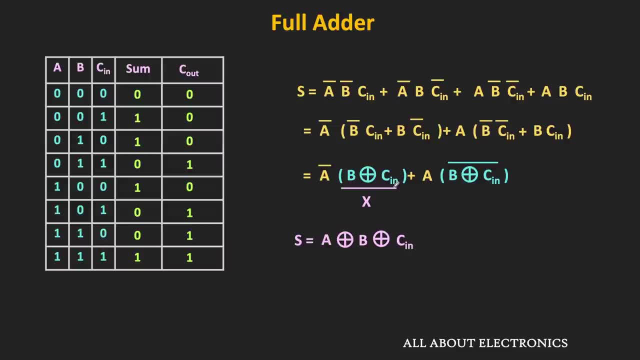 So that is the simplified expression of the sum output. Similarly, let us find the minimal expression for the carry output. As you can see in the truth table, the carry output is equal to 1 for the 4 different input combinations. And this is the expression of the sum output. 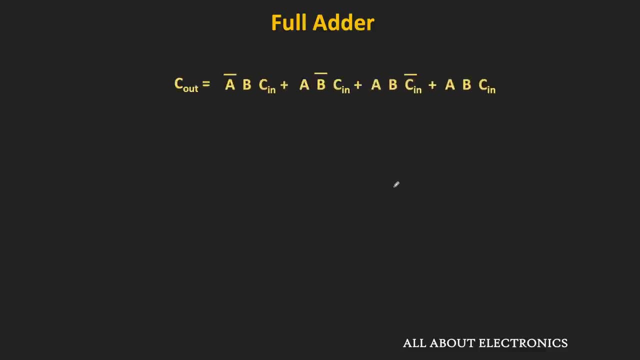 the carry output. So now we can find the minimal expression using the K-Map, And for that, first of all, let us write down all the mean terms in the K-Map. So here this: a, bar, dot, b, dot, cin corresponds to mean term m3.. 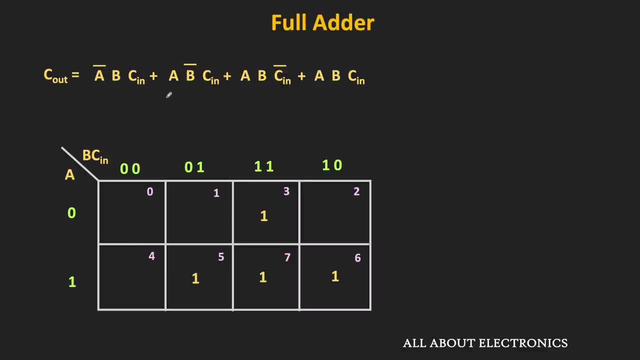 Similarly, this a dot b bar, dot cin, corresponds to mean term m5.. Likewise, this a dot b, dot cin bar corresponds to mean term m6, and this a dot b, dot cin corresponds to mean term m7. So here we can make the group of these m5 and m7. 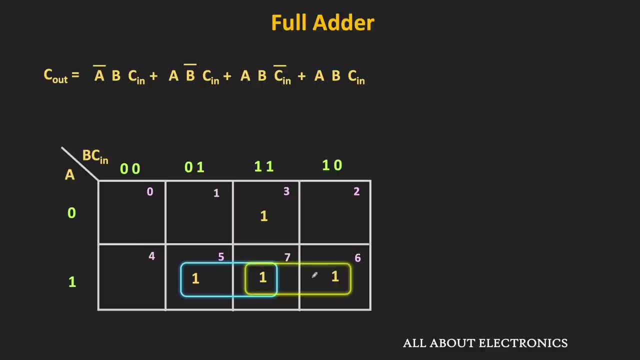 And similarly we can also make the group of m6 and m7. And likewise we can also make the group of this m3 and the m7. So here this group corresponds to b dot cin. Similarly this group corresponds to b dot cin. 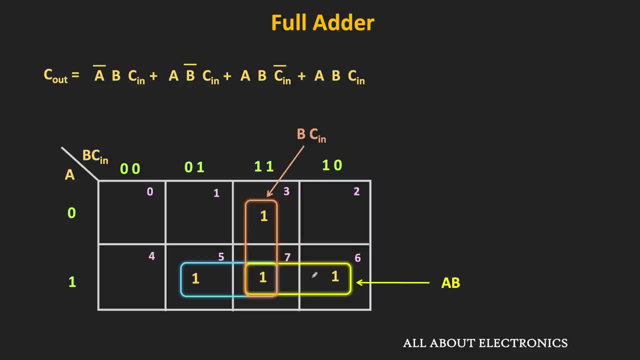 this group in the yellow color corresponds to ab, while this group in the blue color corresponds to asin. So if you see the overall minimized expression for this carry output, then it is equal to ab plus bsin plus asin. Apart from that, we can also write the cout in the different way. 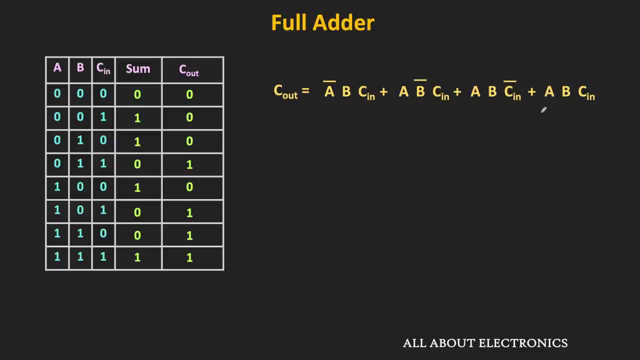 So in this expression, if you see the last two terms, then this ab is common, So let's take it outside. Similarly, in the first two terms this sin is common. So if we take this sin outside, then in the bracket we will have ab plus ad and it. 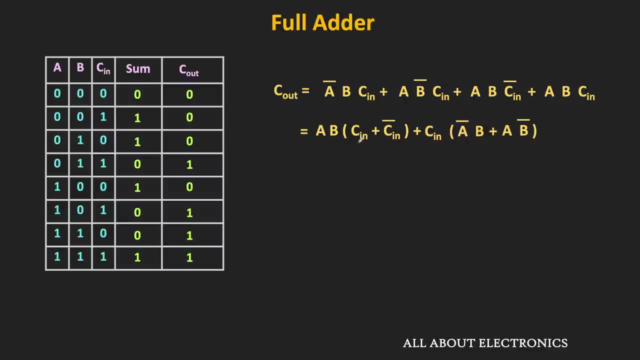 corresponds to ax or b. Similarly, in this first term this sin plus sin bar is equal to 1.. That means we can write this expression as ab plus sinax or b. So that is another way of writing the carry output. 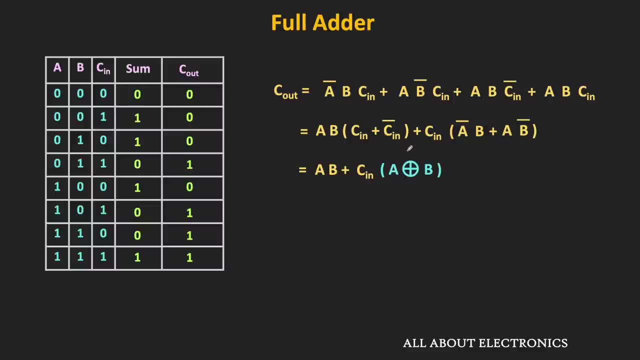 Well, why we have written this expression in this fashion will get clear to you very soon, but this is the second way of writing the output cout. Apart from that, this carry output can also be written as ab plus bsin plus asin. 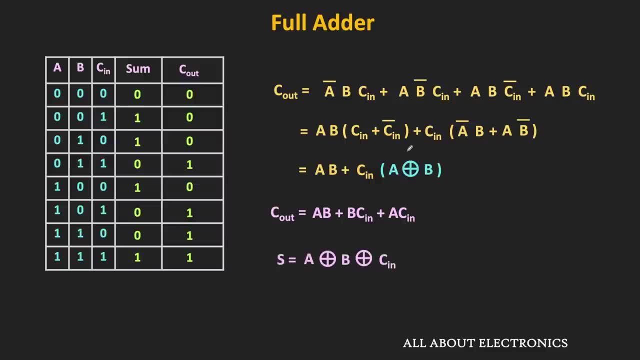 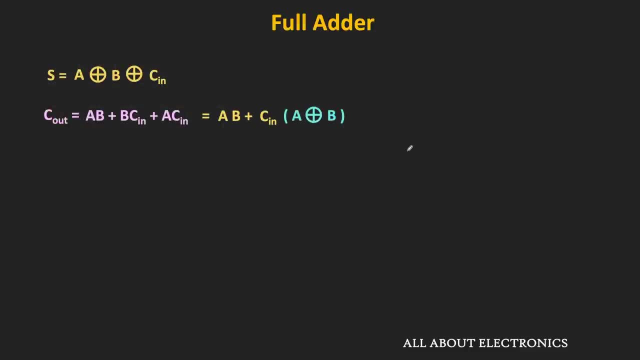 And the sum output can be written as ax or bx or sin. So, Based on this boolean expression, let us see the logical circuit of this full adder. So first, this sum output is equal to A XOR B XOR CIN, So it can be implemented using the two XOR gates. 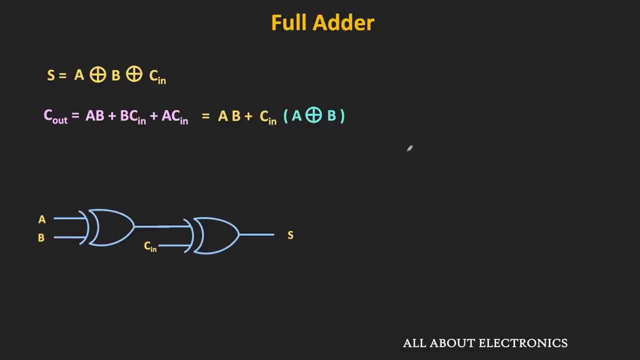 So the output of the first XOR gate is equal to A XOR B and it can be given as an input to the second XOR gate. And the second input to the second XOR gate is equal to CIN, So the output of the second XOR gate will be equal to A XOR B- XOR CIN. 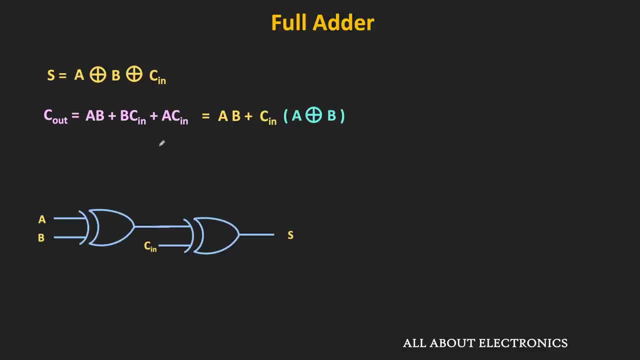 Similarly, from this boolean expression, the COUT can be implemented using the three AND gates and one OR gate. So this is the logic circuit of the full adder. Now if you see the second expression of the COUT, then it is equal to AB plus CINAXORB. 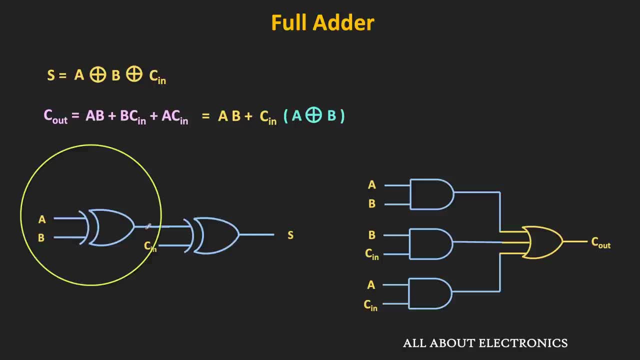 Now, if you see this portion of the circuit, Then we are already generating this AXORB. So using the part of this circuit also, we can generate this carry output. So this is the another way of generating the COUT. So here the output of the first XOR gate is applied to the AND gate. 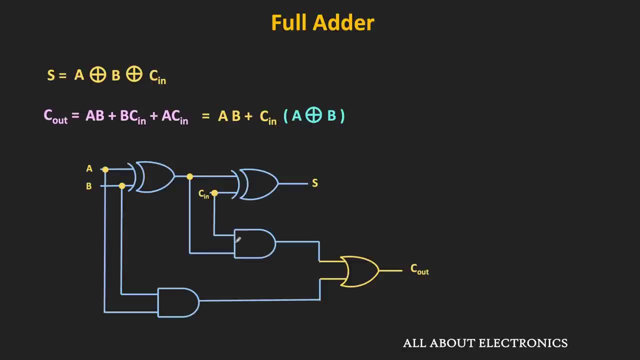 And the second input to the AND gate is equal to CIN. That means the output of this AND gate is equal to AXORBCIN. Now, using the second AND gate, This ab is generated, And using this OR gate, the output of the two AND gate is logically OR. 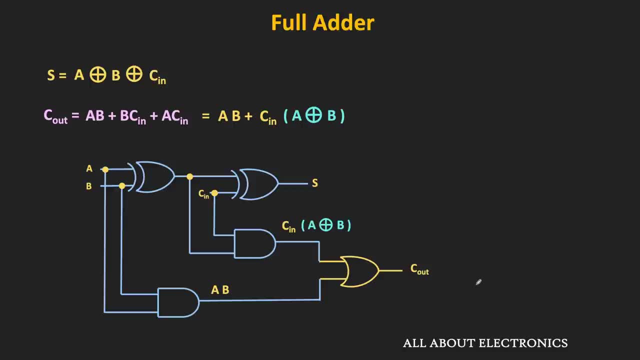 And this is our output cout. So this is the another way of generating the cout. And here, if you closely observe, then this XOR gate and the AND gate is nothing but the half adder. Similarly, this XOR gate and the AND gate forms the second half adder. 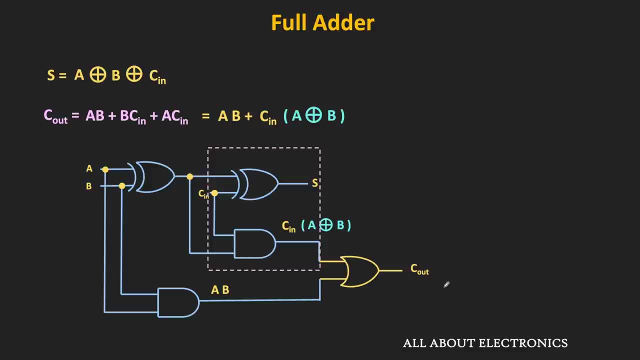 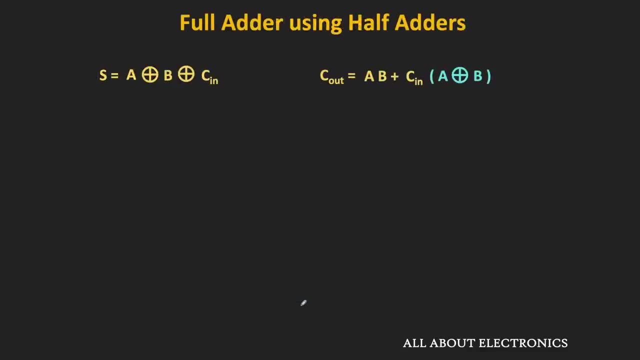 So, using the two half adder and one OR gate, we can generate this full adder. So let's see the same thing from little different perspective. So we know that the half adder consists of one XOR gate and one AND gate. So instead of representing it with the logical circuit, we will represent it with this half. 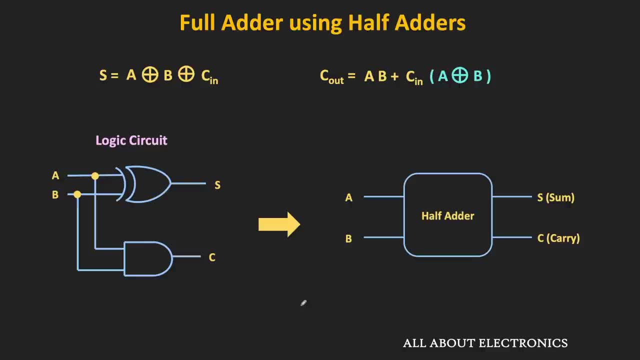 adder block, But just assume that inside it it consists of one XOR gate and one AND gate. So if A and B is the input to the half adder, then the carry output is equal to ab, while the sum output is equal to AXOR B. 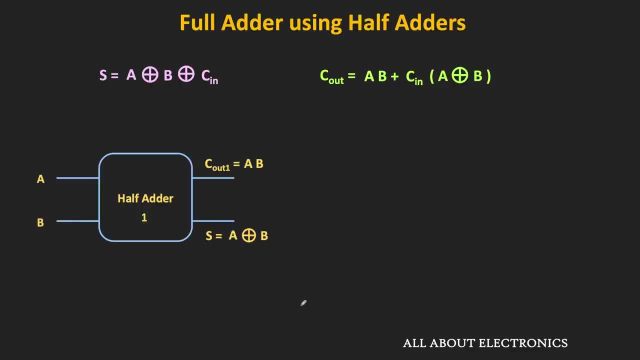 Now the sum output is applied as an input to this second half adder, And the second input to this second half adder is equal to cin. So the sum output of this second half adder is equal to Axor BXOR Cin. 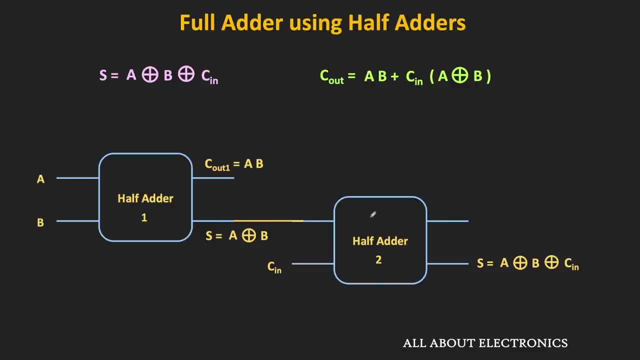 And similar to the ab. Now, after the first half adder, we are already getting this AB. So using one OR gate we can perform the logical OR operation of these Cout1 and Cout2.. And that is our carry output of this full adder.